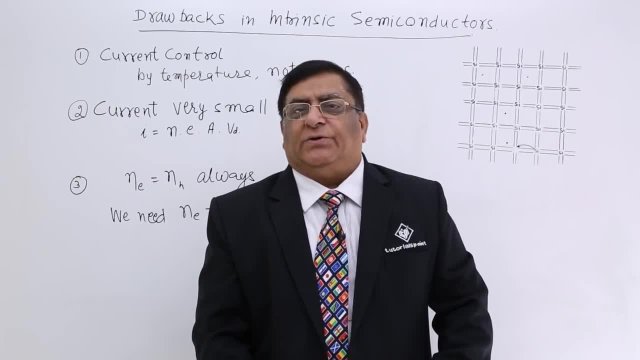 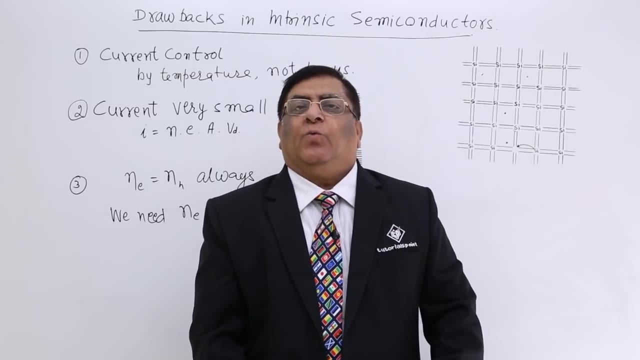 The intrinsic or 100 percent pure semiconductors are not fit for making devices, Devices which we are going to study, which are diodes, transistors and other devices. Why these semiconductors, which are so pure, cannot be used? This is because of the three reasons. See the reason. 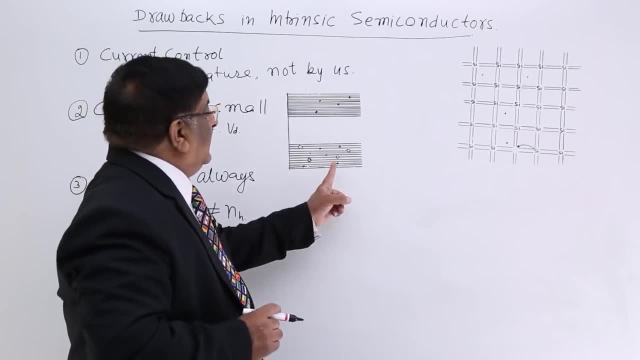 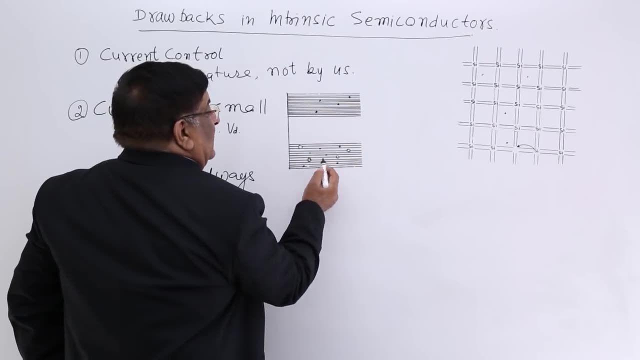 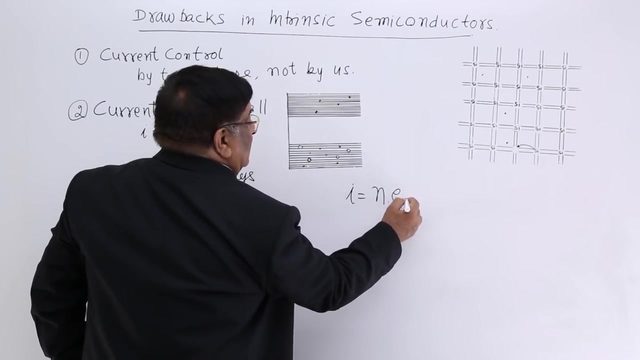 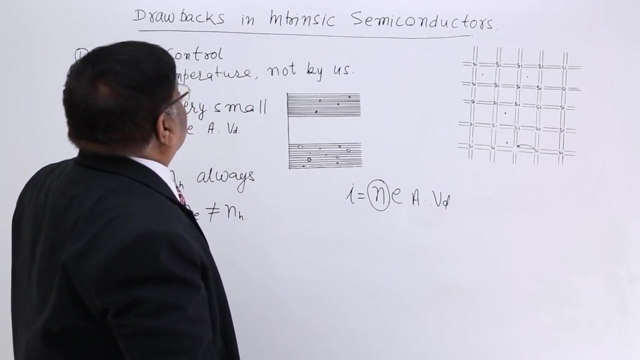 one is that here, who is responsible for current Answer, the number of free electrons and the number of holes? Because we know the formula for current is N, E, A drift velocity and this is number of charged particles. Now in this, who is controlling the number of charged? 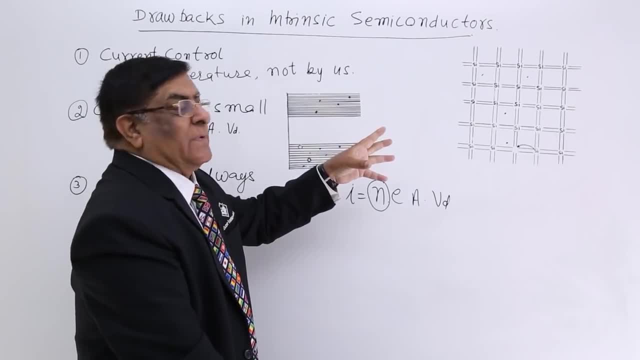 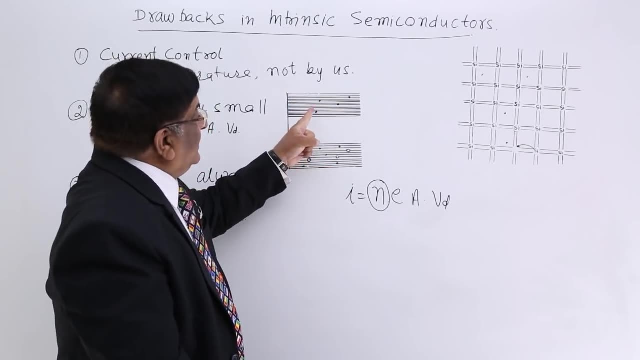 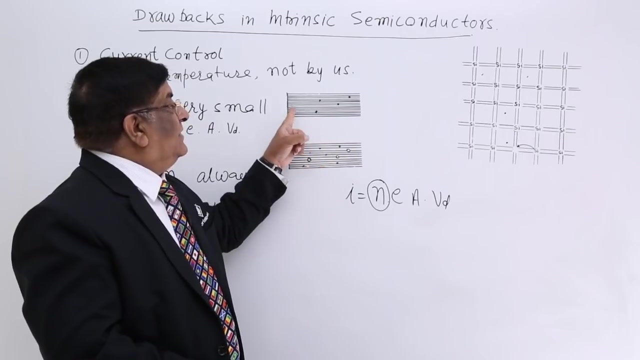 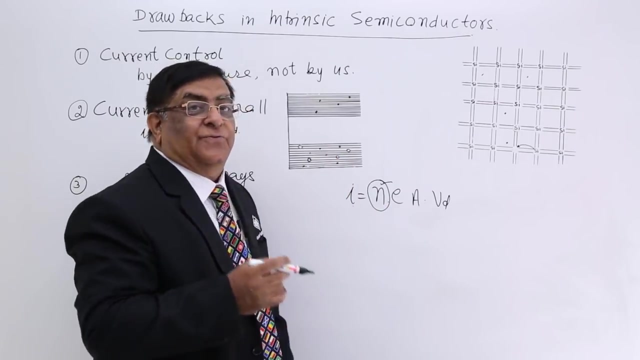 particles Which are responsible to flow. If the temperature of this semiconductor increase, then these electrons numbers will increase. Some more electrons will get energy. they go here and the number of conduction electron will increase. the current will increase. with what temperature? Now I have made a computer which gives certain values. 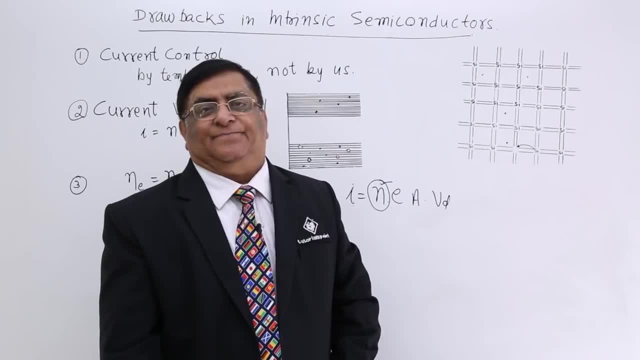 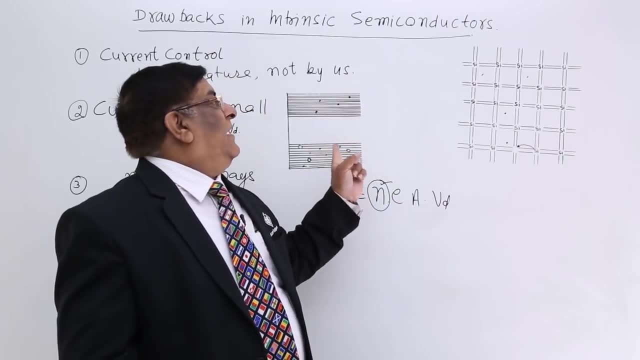 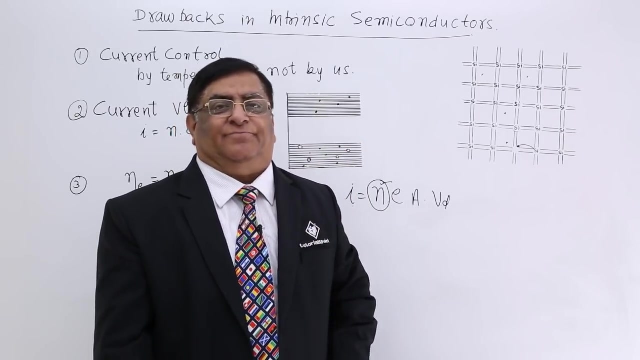 Which gives certain result based on the current. If it is goes to a hot country and their temperature is high, then the number of electrons will be more here and that current will increase. The results will not be same. But that is not under my control. that is under the control. 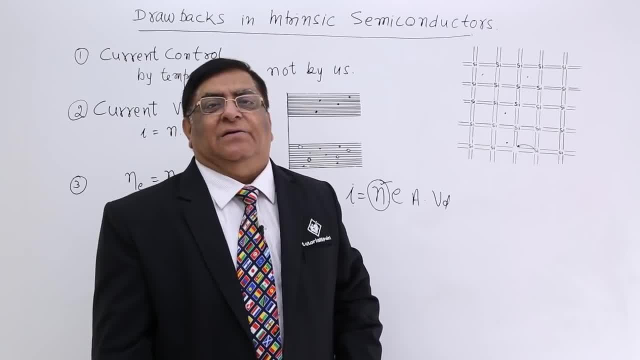 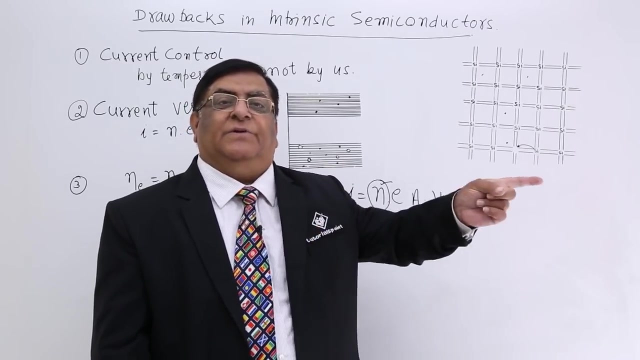 of temperature, And this is something which forbids me to make a device. So I am going to make a device, So I want that control of electric current. How much will be the electric current that should be with me, not with the temperature? This is the one problem. 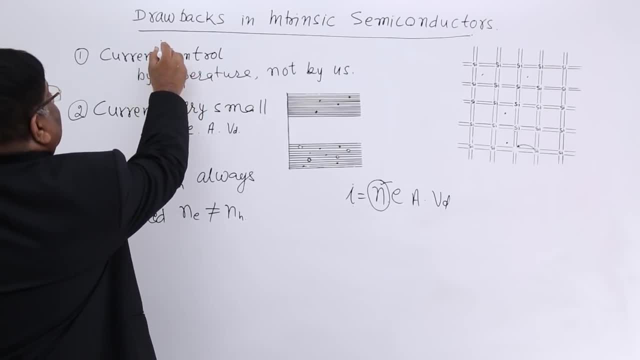 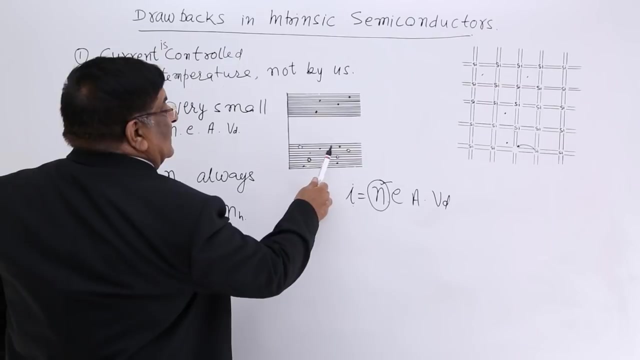 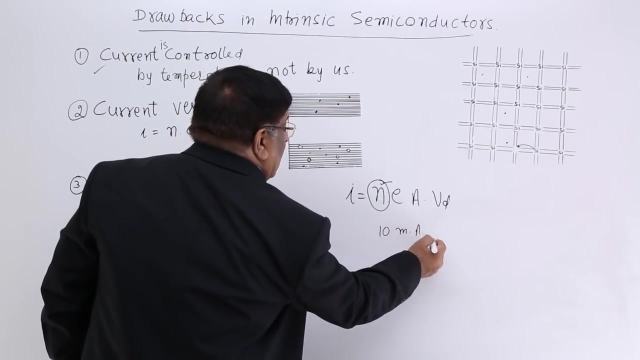 that the current was controlled. Current is controlled by temperature, not by us. Now, second, current is very small. Again, at room temperature certain electrons are there may be plus minus 10 degree. Even these number of electrons can make a limited current. Suppose this current is 10 milli amperes. 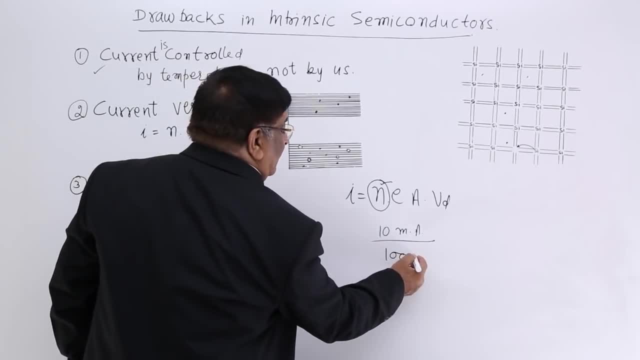 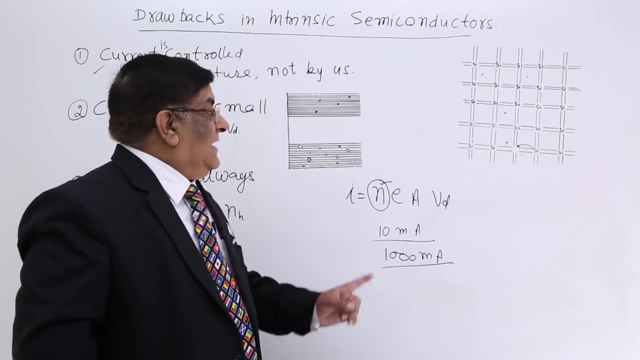 I want to make a device which has got 1000 milli amperes. I need 1000 milli ampere to flow through semiconductor. Then how to make this 10 milli ampere? I want to make a device which has got 1000 milli amperes. I need 1000 milli ampere to flow through semiconductor. 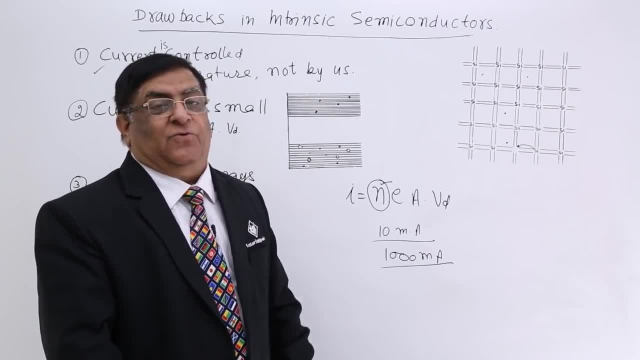 That means which of milligram be 1000 millias? Then what is Schwe Arri living on 1 milli ampere? 1000 milli amperes? I have no way. So this current is not sufficient for many. 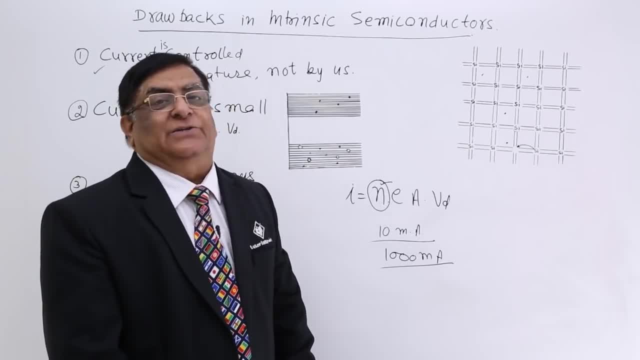 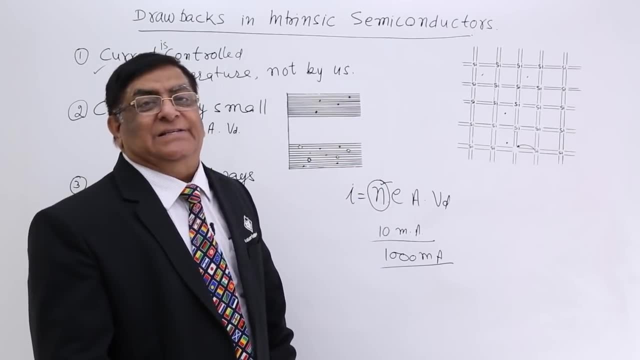 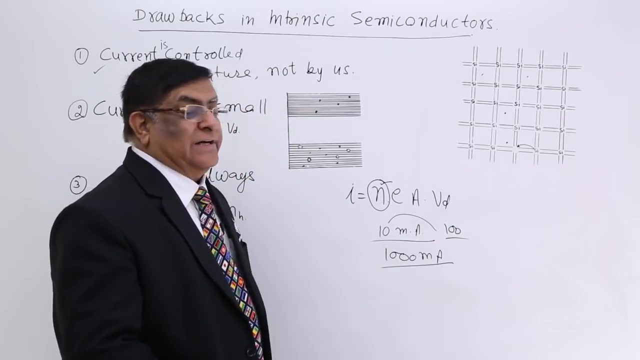 devices which need high current, And that control is not with me. I cannot keep it at a very high temperature At all the places, and even high temperature will make it 10 times higher, But I want this 100 times higher. That is not possible. 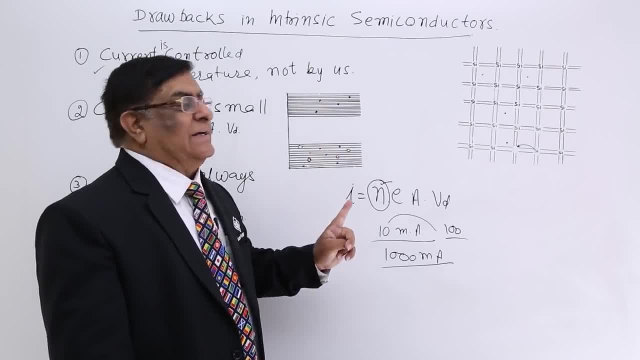 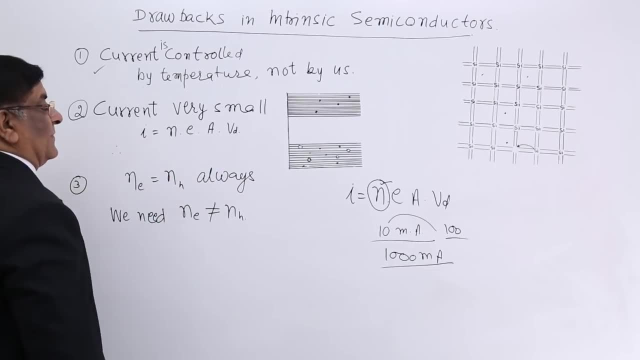 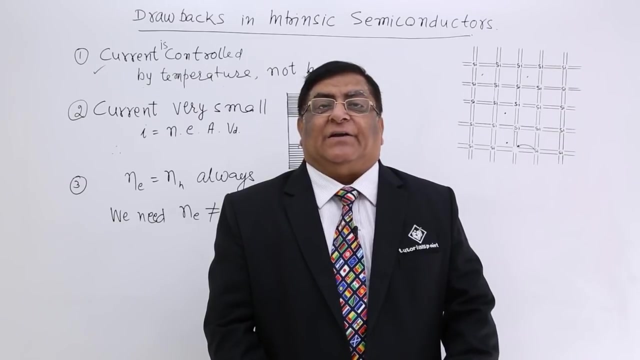 the current in this intrinsic semiconductor is limited. Current is very small, therefore not suitable. Third feature is that number of electrons and number of holes both are equal to each other. When they are equal to each other, then this feature also is not suitable for making devices. When we want to make devices that I will show you in the next lecture, then 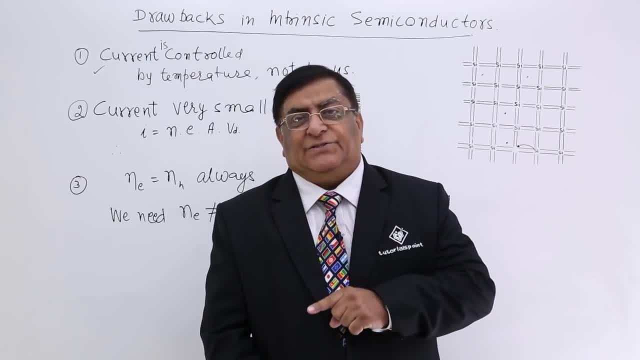 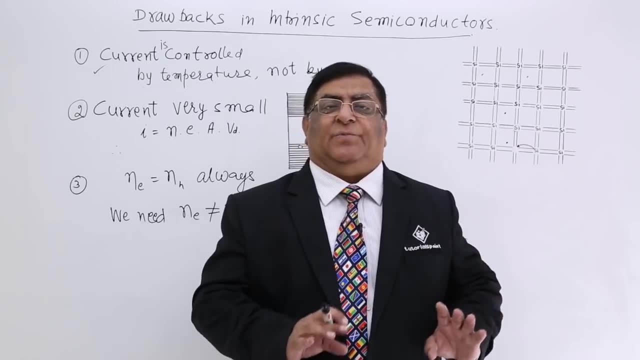 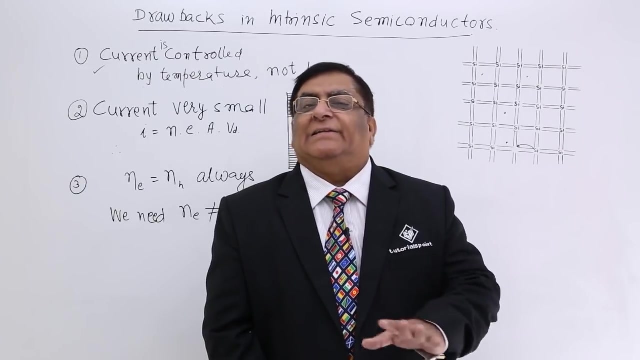 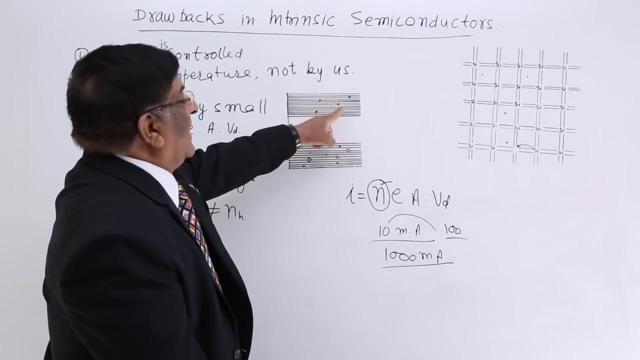 we need: either Ne should be very large or NH should be very large compared to each other, one should be less and one should be large, and then only our design of device will work. and that is not possible in intrinsic, Because here, whatever electrons are leaving this, are going here. So Ne is always equal to NH. So these are the three problems Current.